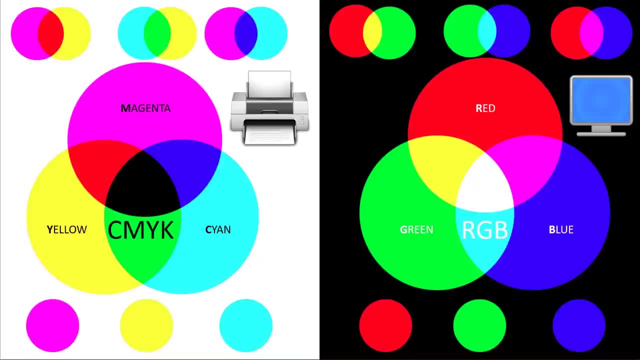 as well as what that means. So CMYK is used in printing, which you may have noticed. a printer has ink cartridges labeled cyan, magenta, yellow and black CMYK. However fun fact, the K technically stands for key. 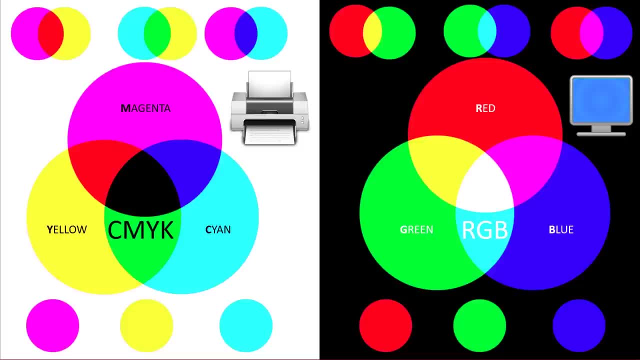 not black, like many people rather reasonably assume. Now we'll come back to CMYK in a second, but first let's go over RGB right now, which is an additive color. This is the model that the computer screen you're watching this video with right now is using, So let's talk about how it works. 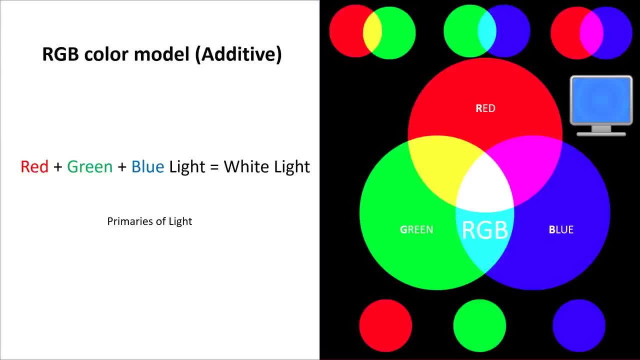 The RGB additive color model works in terms of light. So basically, red added to green added to blue equals white Additive. Let's look at a visual representation of what this would look like in real life. Here we have red light, green light and blue light all shining on a dark wall. The result looks: 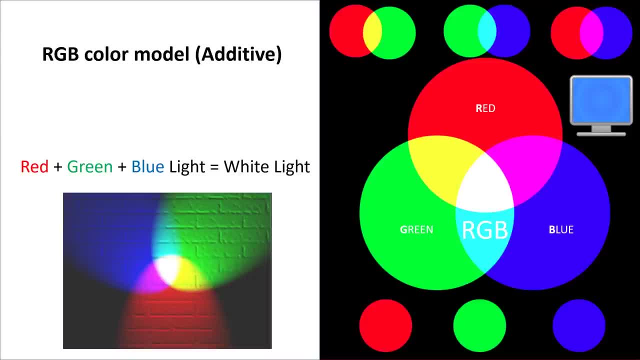 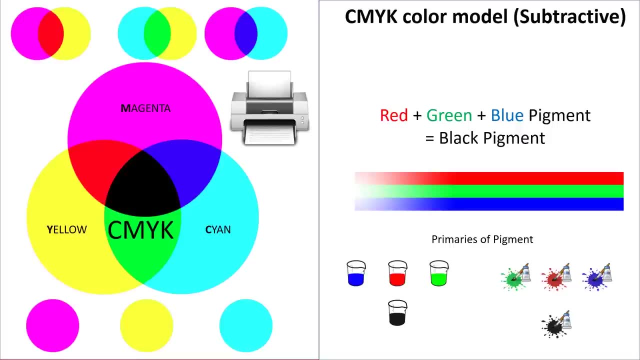 pretty similar to what we had before, as opposed to CMYK. The CMYK subtractive color model works in terms of pigment. In this model, combining red, green and blue gets us black. So, unlike light, which is additive and adds up to white, pigments are subtractive and combine into black. We see: 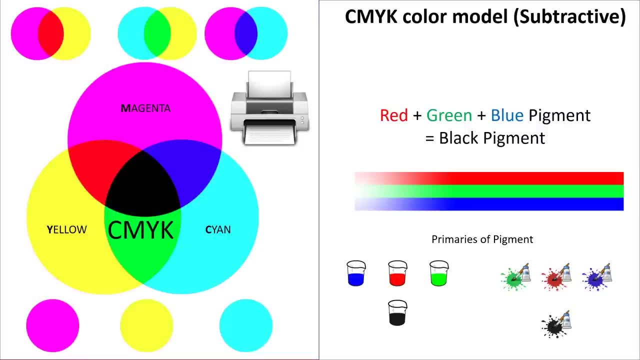 subtractive color mixing every day in things like ink and paint. For example, if you mix red, green and blue, you'll get black. Let's talk about why this is Ok, so we're going to put ones next to our. 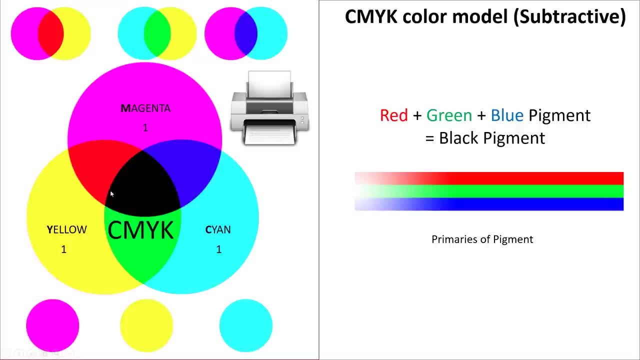 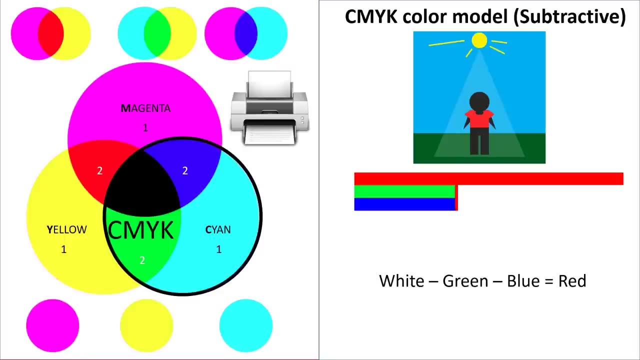 three primary pigment colors: cyan, magenta and yellow. Next, we're going to put twos next to our secondary pigment colors and we'll explain why we did this in a moment. But first an example. Say you're wearing a red shirt when white light, which we now know, is made up of red, green. 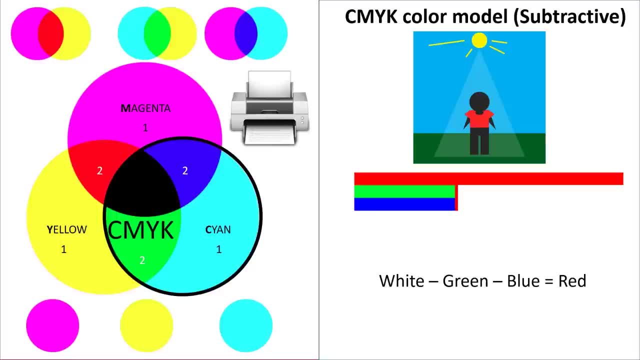 and blue light hits your shirt, What happens is your shirt absorbs all the color that hit it, except for red. The shirt reflects the color red, and so that's what we see. Think of it almost as a barrier which only lets the color that it happens to be pass through. Now for clarification, let's.